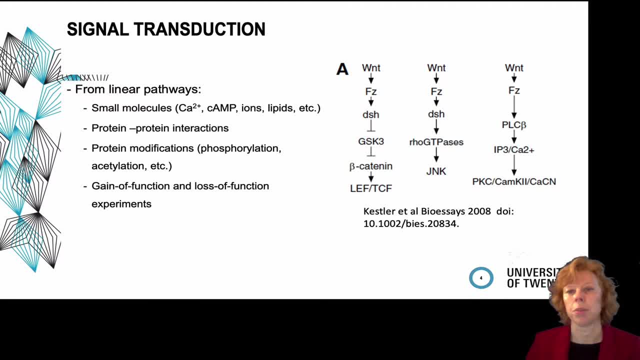 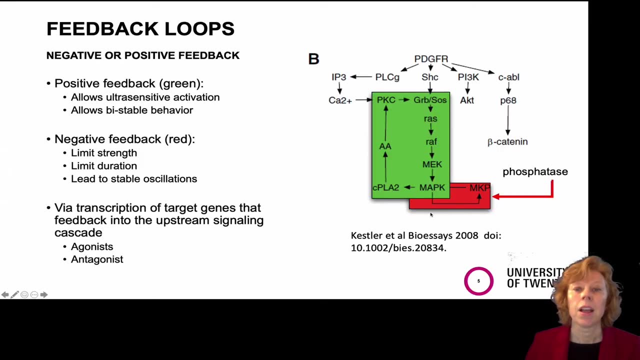 by inducing a strong and visible genetic phenotype. Many experimental methods are available to investigate individual proteins, even in multiplex, so that changes in activity or modification state can be quantified. Let's take a look at some examples of signal transduction research. 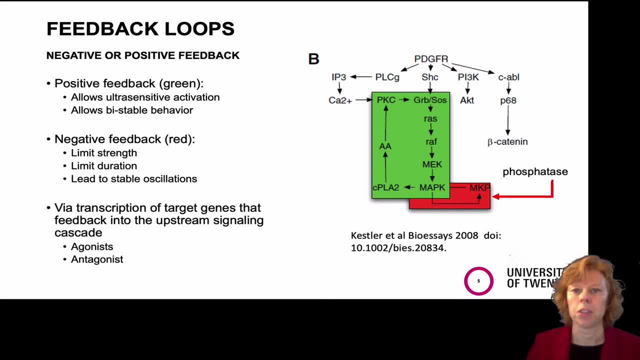 Linear cascades might be enhanced by inclusion of feedback loops. Feedback loops can be positive or negative. Feedback loops play an important role in modulating the strength and duration of the signal. Phosphatases can limit the signal strength and duration by inactivating specific kinases. In addition, feedback loops are known. 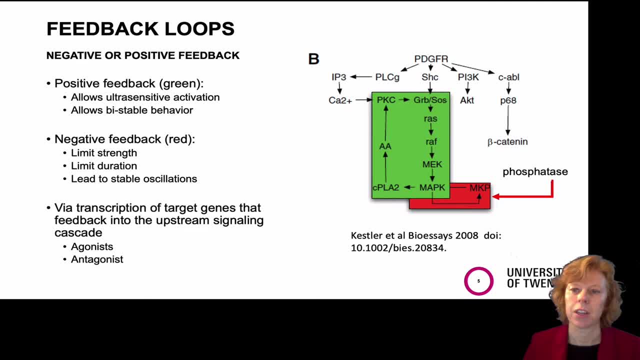 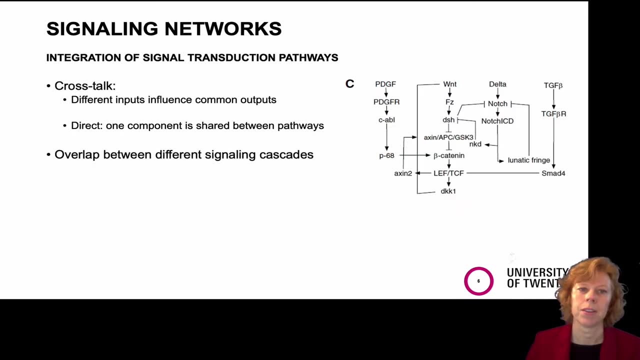 to function through activation of genes that can regulate the upstream signaling cascade. These include agonists that activate the pathway, such as ligands, or antagonists that block the receptors by preventing ligand binding or receptor activation. We now know that signal transduction pathways are integrated into networks. These networks 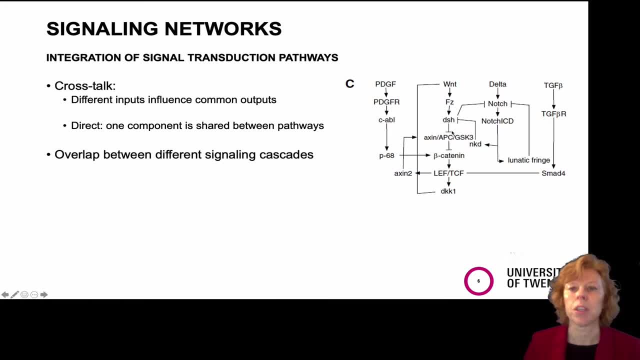 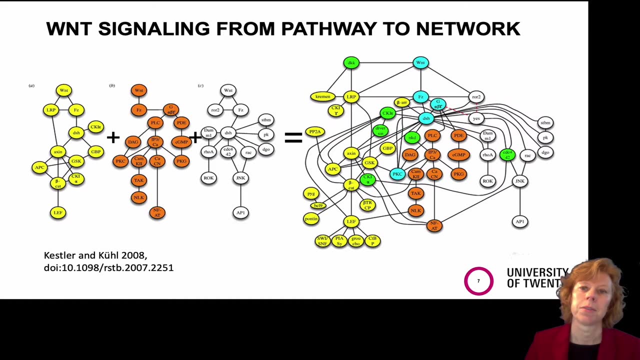 are a result of signaling crosstalk, in which different inputs influence common outputs. This is called direct. when a single component is shared between different pathways, There is great overlap between different signaling cascades, which makes it hard to predict a cellular response. To illustrate what networks look like, we look at the wind signaling pathway- The wind. 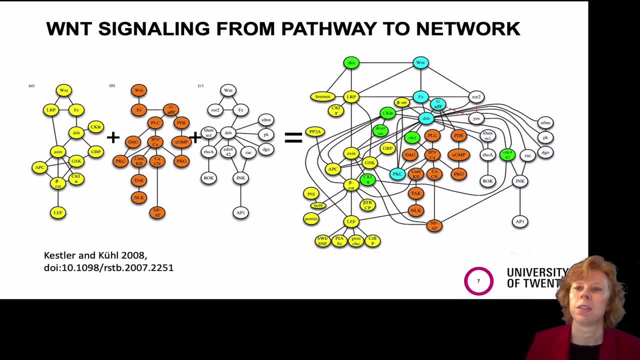 pathways are important during development and tissue maintenance. There are 19 wind ligands described and over 10 frizzled receptors in higher vertebrates alone, which prompted the question whether wind ligands activate identical pathways and are thus redundant, or if different signaling pathways can be activated by the same wind ligands. 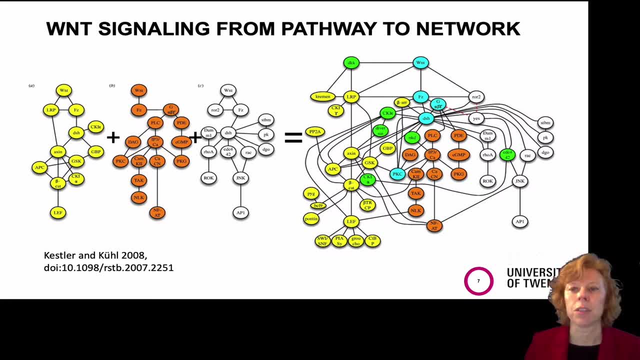 And indeed many labs have found that wind ligands can activate different pathways – the wind beta-catenin or canonical pathway, and the nonical, wind calcium and wind junk pathways. Wind signaling pathways were considered to be individual pathways. Kessler and Kuhl proposed in 2008 that the individual pathways overlap and form a wind. 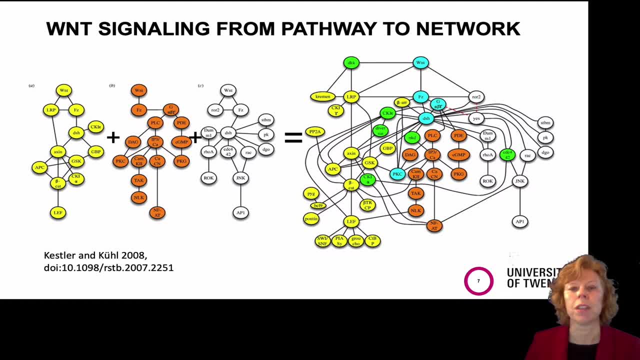 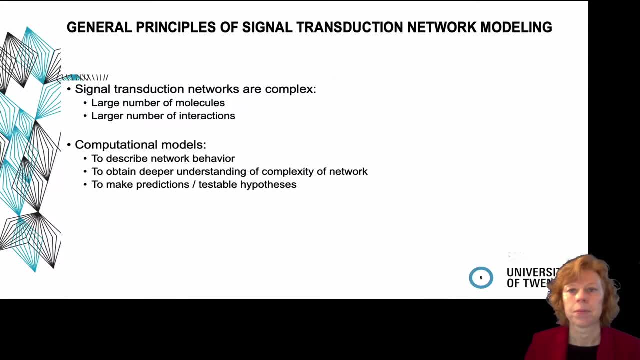 network in which combinations of multiple wind ligands and wind receptors dictate cell function. Signal transduction networks are complex due to the large number of interactions and non-linear topologies. To understand cell function, computational models are used to describe network behavior, to obtain a deeper understanding of the complexity of the network and even to make predictions. 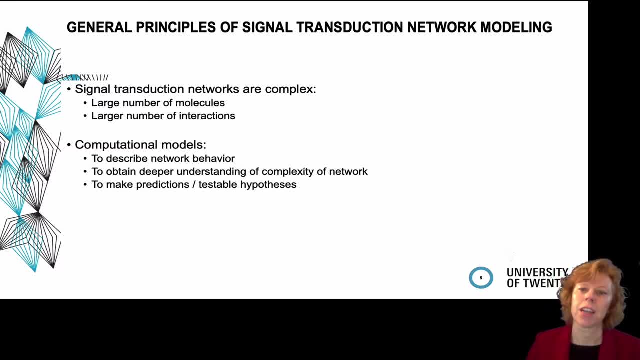 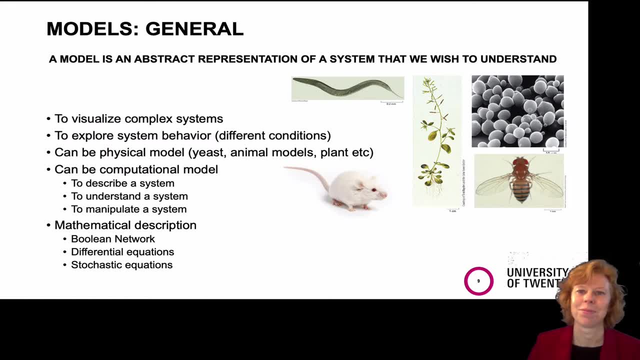 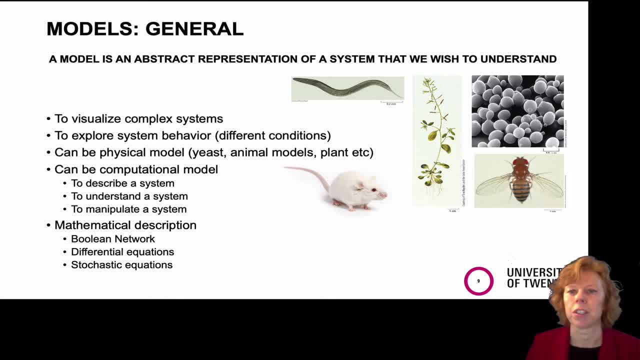 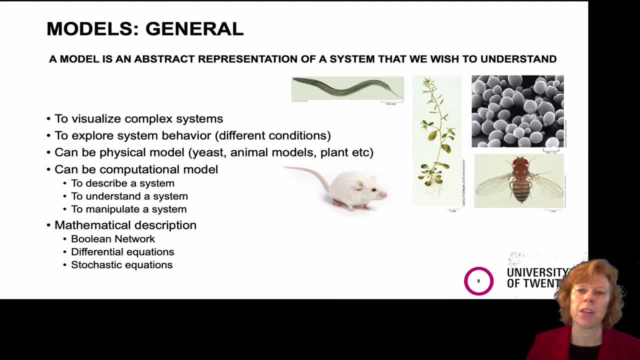 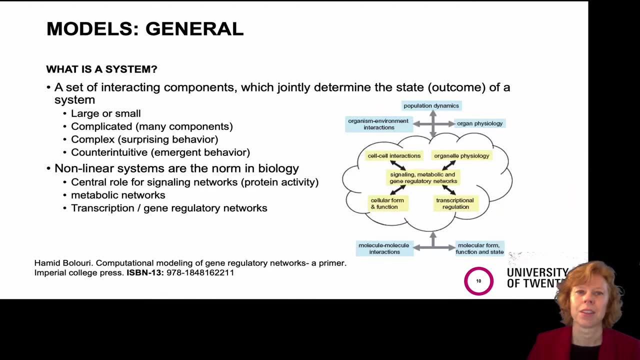 computational model that is used to describe, understand and manipulate a system. There are various mathematical descriptions used for modeling. The most known are Boolean networks, differential equations and stochastic equations. So what is a system? It is a set of interacting components which jointly 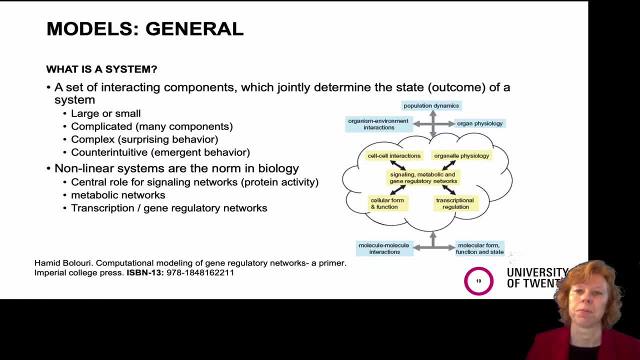 determine the state or the outcome of a system. A system can be large or small. complicated meaning they have a lot of components, and also complex, meaning they exhibit behaviors that are surprising or difficult to understand. Some system behaviors can be so complex as to be counterintuitive. This type of behavior 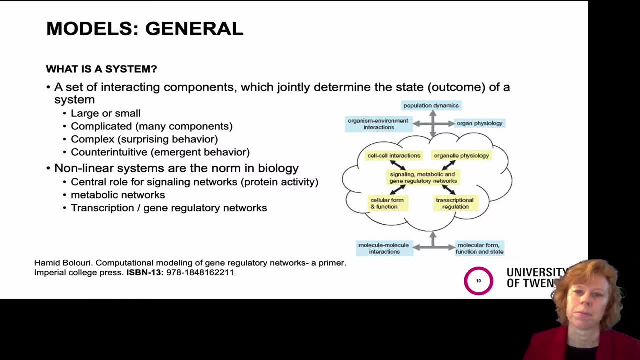 is sometimes referred to as emergent behavior. In biology, nonlinear systems are the norm. Biological systems exist and can be studied at many levels of resolution. However, there is a central role for signaling networks, as depicted in this picture, because it plays such an. 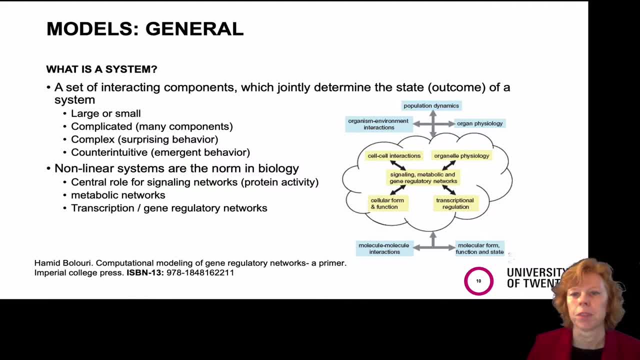 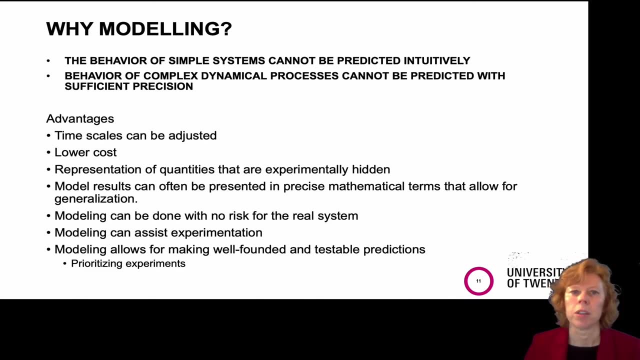 important role in regulating all the cell function. Also, metabolic networks and transcription or gene regulatory networks are often described by computational models. Why do we need modeling? We need it because the behavior of simple systems cannot be predicted intuitively and from experience. The behavior of complex, dynamical processes 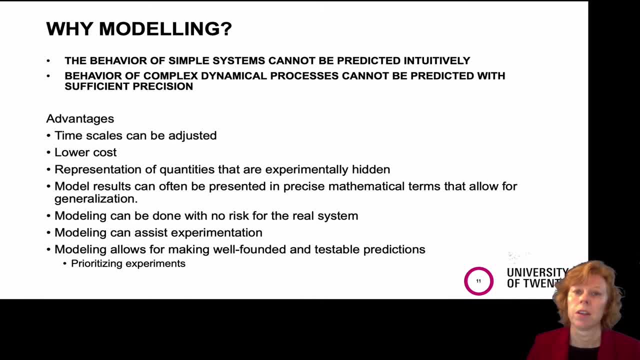 cannot be predicted with sufficient precision. For both prediction and explanation of processes, one needs a model. There are many advantages to using a computational model. Timescales can be adjusted, The costs of computation can be adjusted. The cost of computation can are much lower than those of wet lab experiments. a model can represent quantities that are 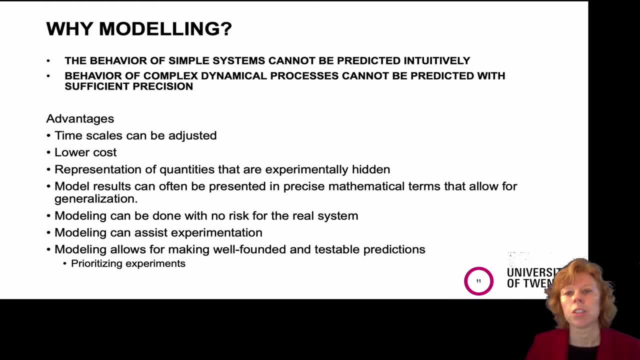 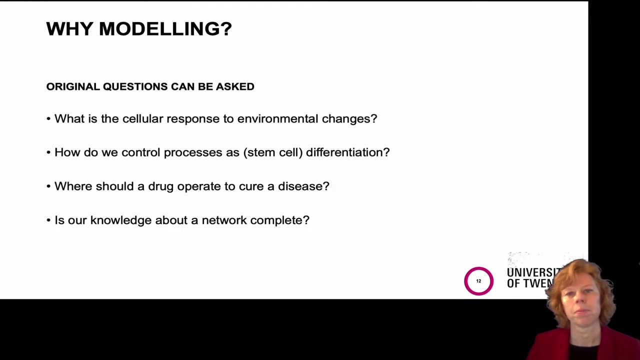 experimentally hidden model results can often be presented in precise mathematical terms. that allows for generalization and quantification. modeling can be done with no risk for the real system and can exist experimentation and allow for making well-founded and testable predictions, which in turn allows prioritizing experiments. 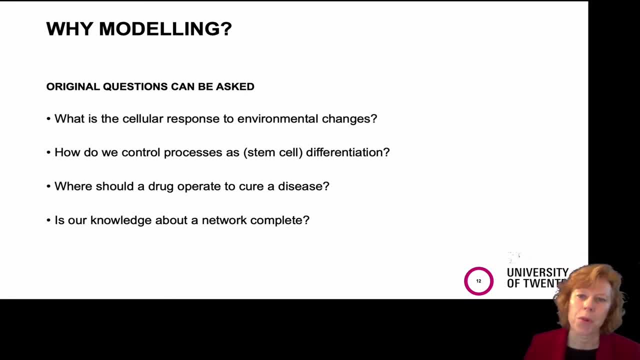 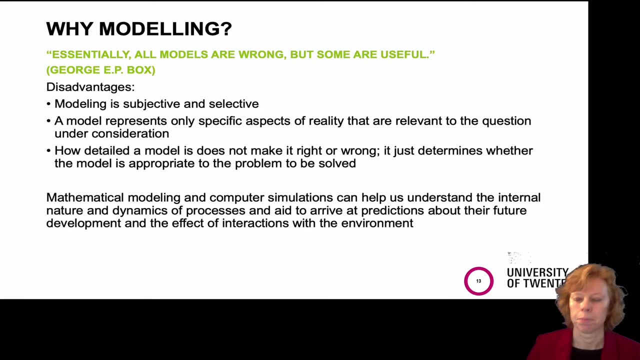 Many relevant and original questions can be asked. for example, what is the cellular response to environmental changes and how do we control processes as, for example, stem cell differentiation? Where should a drug operate to cure a disease and is our knowledge about a network complete? 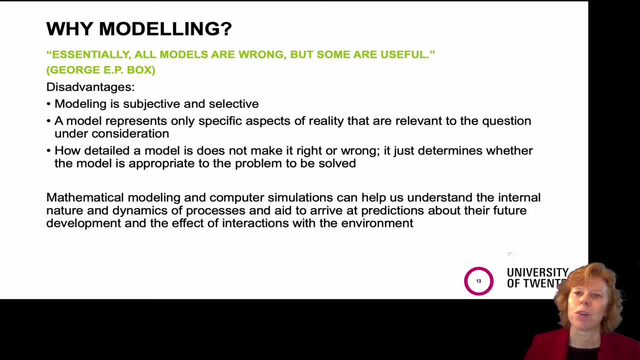 So let's look at some of these questions. A popular quote is George Box's remark that all models are wrong, but some are useful. And indeed it's good to keep in mind that there are disadvantages to modeling. For example, modeling is subjective and selective, since the model builder will make choices. 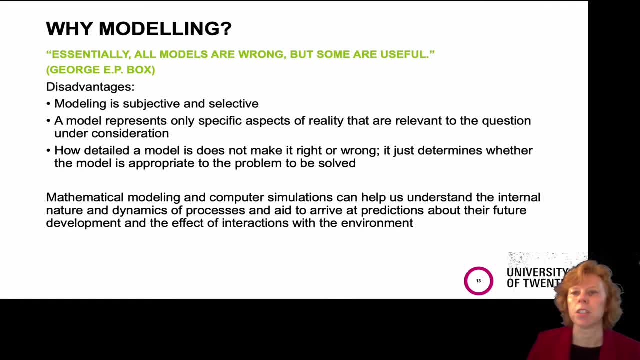 and these choices are based on the model builder's experience and knowledge. A model only represents specific aspects of reality that are relevant to the question under consideration. Models can be broad or detailed, And how detailed a model can be depends on the model A model is does not make it right or wrong. 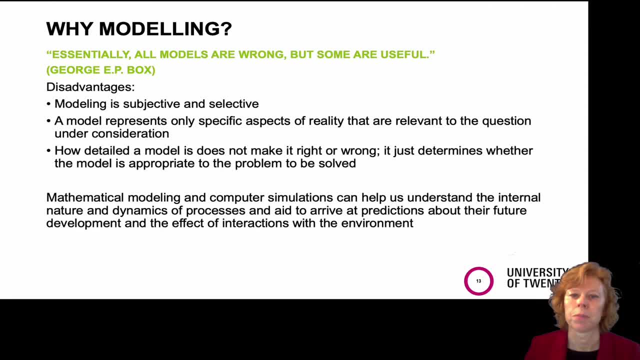 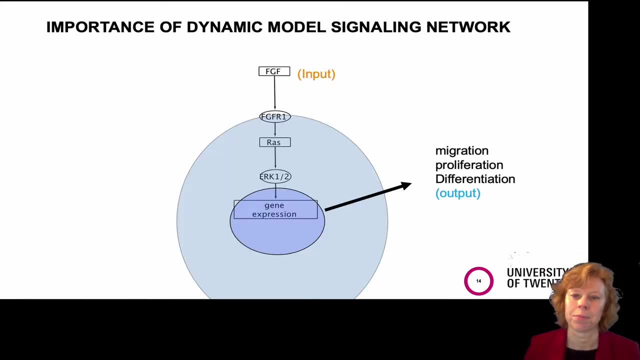 It just determines whether the model is appropriate to the problem to be solved In the end. mathematical modeling and computer simulations can help us understand the internal nature and dynamics of processes and aid to arrive at predictions about our future development and the effect of interactions with the environment. 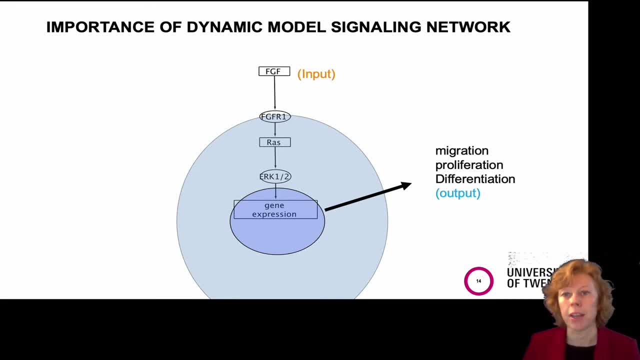 We'd like to illustrate the importance of dynamic models. If you take, for example, an input which could be a growth factor and an output which could be gene expression, resulting in cell migration or differentiation, traditionally, cellular processes were studied in isolation, out of context in the network in which they 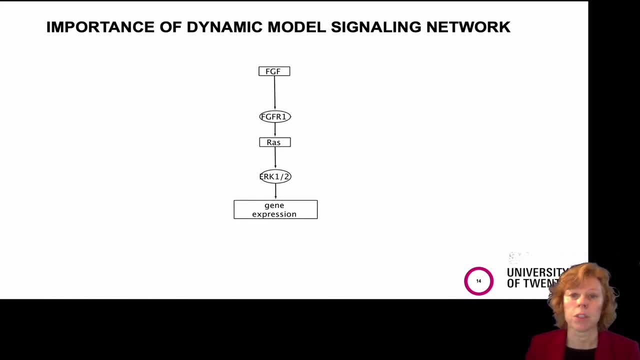 function. Moreover, the processes were described only in a static and qualitative way, as in this example: a static topology of a growth factor pathway To obtain insight into dynamics of processes. one can formalize the network, thereby including activity levels, as is shown by the colors of the network in this example. 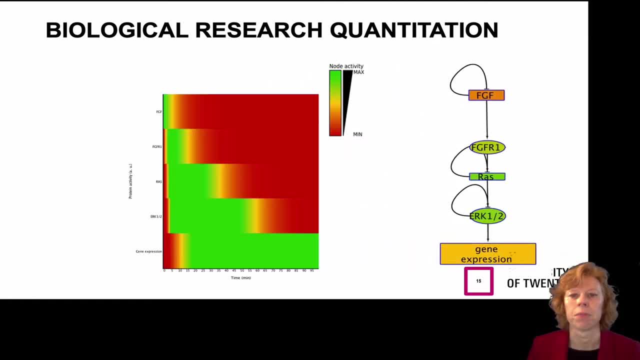 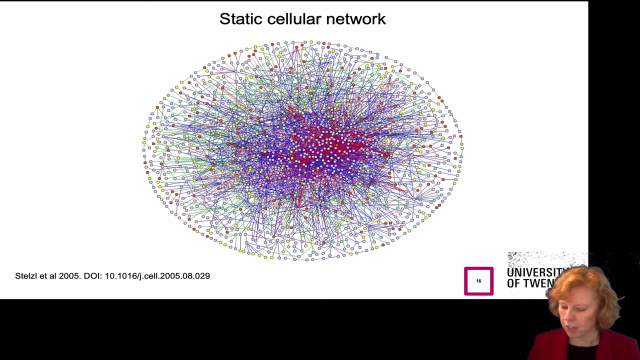 This is the first example. Here we see that activation of the ligand activates the intracellular cascade, which results in activation of gene expression. However, formalizing this single signaling pathway is such an oversimplification that there is loss of reality, Because in reality, at any given point, cells are exposed to many signals that are integrated. 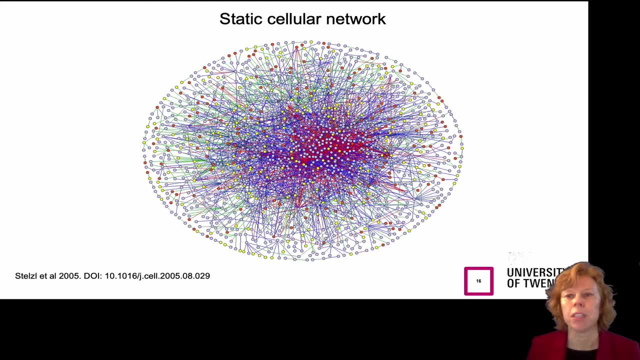 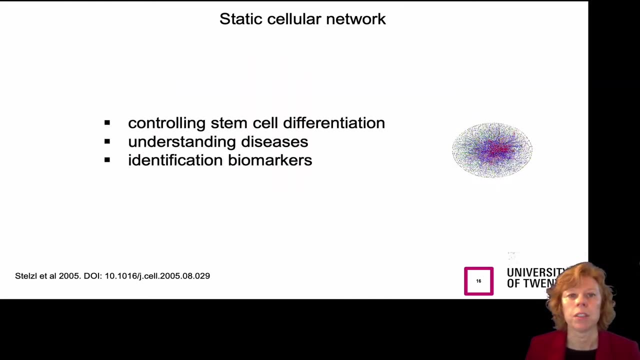 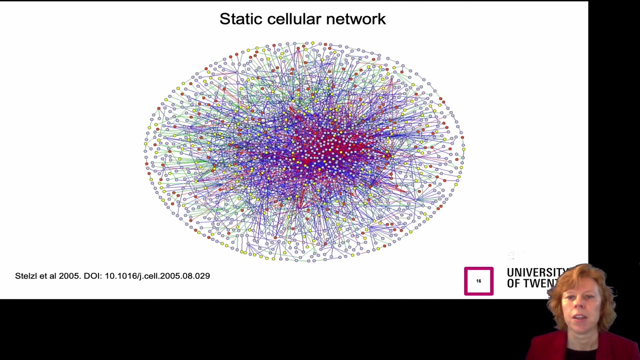 to determine the cell response, as shown in this amazing picture of a proteome that shows thousands of protein interactions in a static representation. Insights into processes regulating cell fate are important for controlling stem cell differentiation, understanding diseases, identification of biomarkers, designing precision therapies. 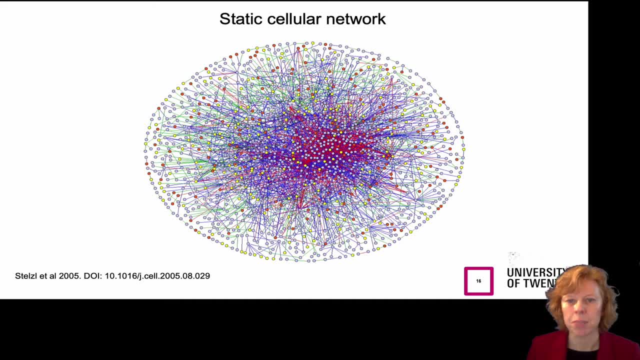 So no empirical testing is possible to test all the interactions in this image. So no empirical testing is possible to test all the interactions in this image. Our brains are simply incapable of integrating, interpreting and prioritizing these complex mechanisms, Which is why you can use mathematical models. 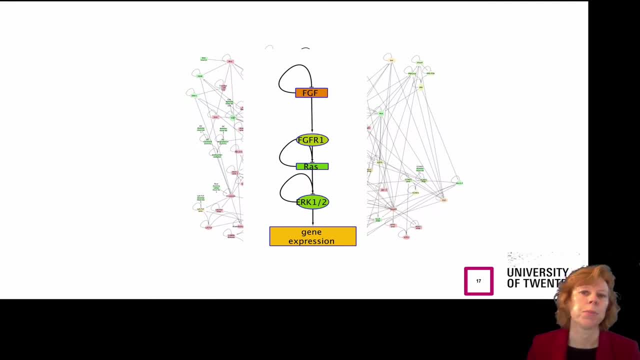 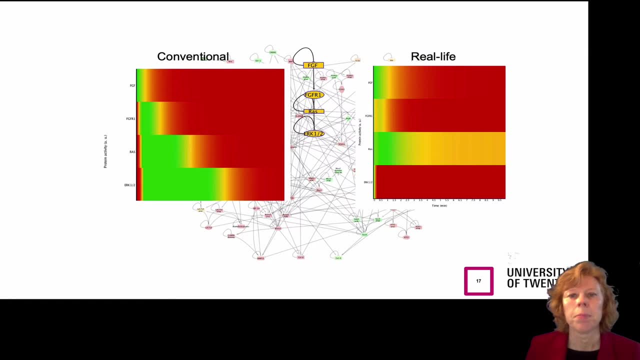 So this simple growth factor pathway will have to be investigated in the context of many other signals. As you can see by the activity plot, investigation of the FGF pathway in context of other relevant signal greatly changes the expected activity profile much more closely resembles the processes in real life. This highlights 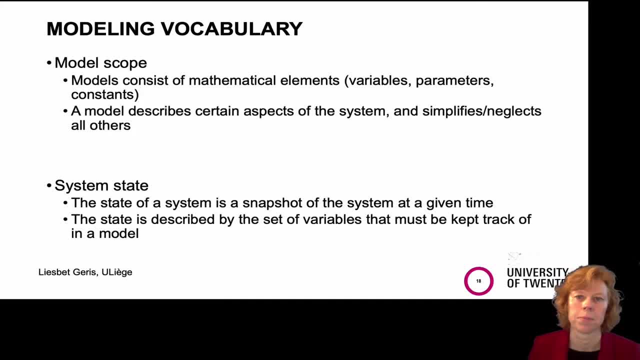 the necessity of studying cellular processes in context. So let's turn to some of the modeling vocabulary that you will encounter reading papers. By model scope we mean the objectives and requirements of the model. A model consists of various mathematical elements, such as variables, parameters and 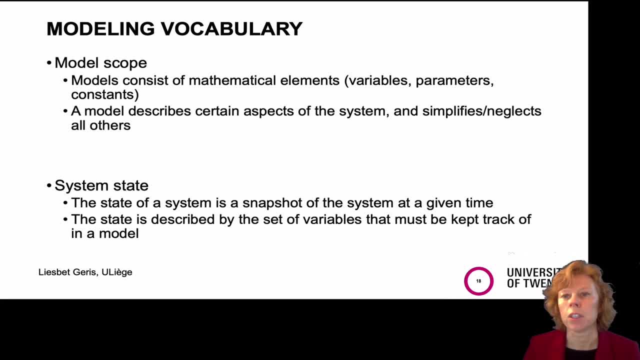 constants. The model is fairly focused, meaning that it describes only certain aspects of the system and simplifies or neglects all others. When we talk about system states, one has to realize that the state of a system is a snapshot of the system at a given time point, and that the state is described by the set. 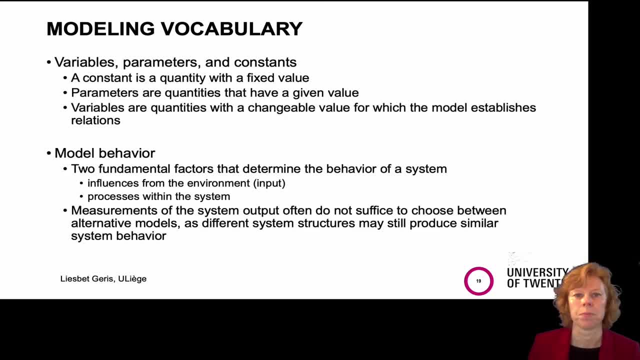 of variables that must be kept track of in a model. You probably know. a constant is a defined quantity with a fixed value. Parameters have an unknown or variable quantity that can have a given value selected for the specific circumstances of the model and in relation to other. 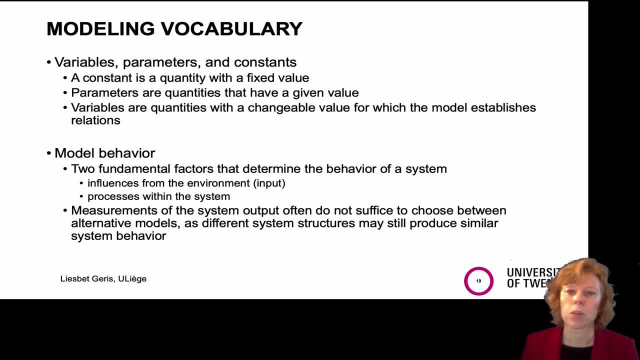 variable quantities in the model. Variables are quantities with changeable values for which the model establishes relations. When we talk about model behavior, we assess two fundamental factors that determine the state of the model: the influences from the environment, inputs and the processes in the system. For example, integrity. In our model, we are concerned about each set ofum. 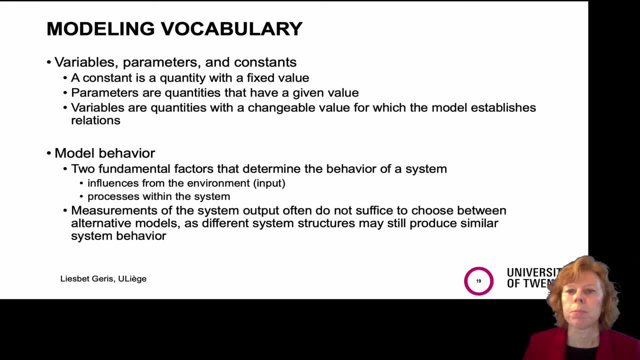 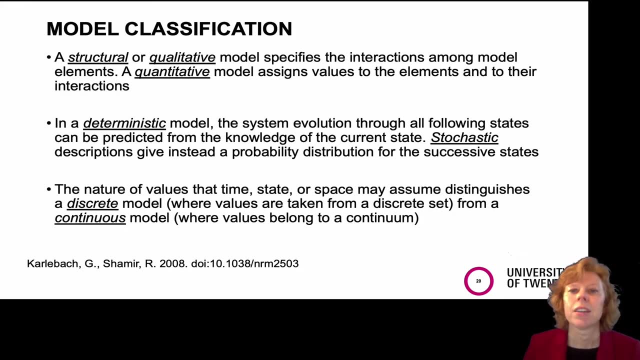 intracellular signalling molecules. When we look at model behaviour, measurements of the system output often are not sufficient for choosing between alternative models, as different system structures may still produce similar system behaviour. There are different types of models: qualitative and quantitative models. A structure or qualitative model specifies the interactions among model elements. 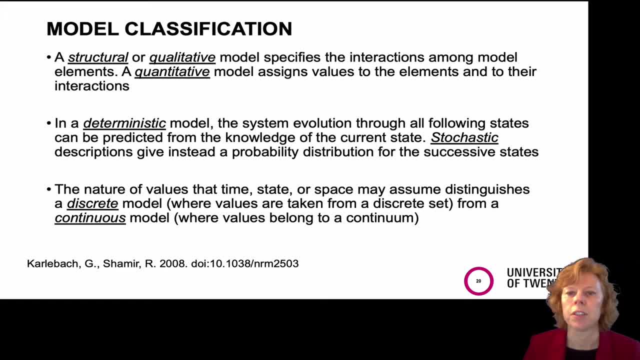 A quantitative model assigns values to the elements and to their interactions. In a deterministic model, the system evolution through all following states can be predicted from the knowledge of the current state. Stochastic descriptions give instead a probability distribution for the successive states. The nature of values that time, state or space may assume distinguishes a discrete model. 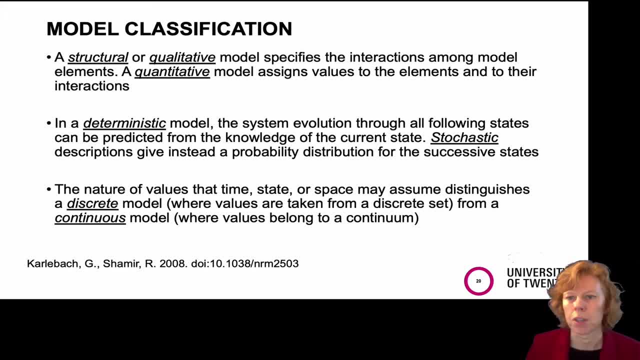 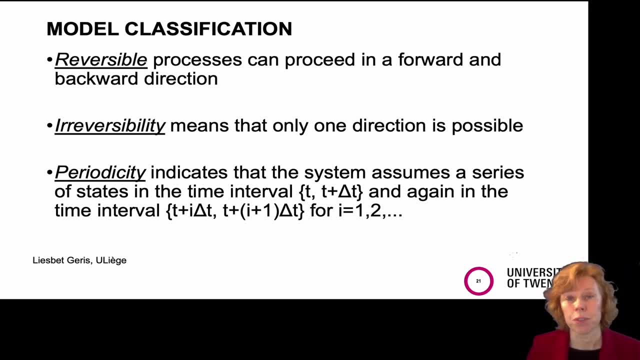 where values are taken from a discrete model. The nature of values that time, state or space may assume distinguishes a discrete model where values are taken from a discrete model. In models, we can have different processes: Reversible processes that proceed in forward and backward direction. irreversible, in which 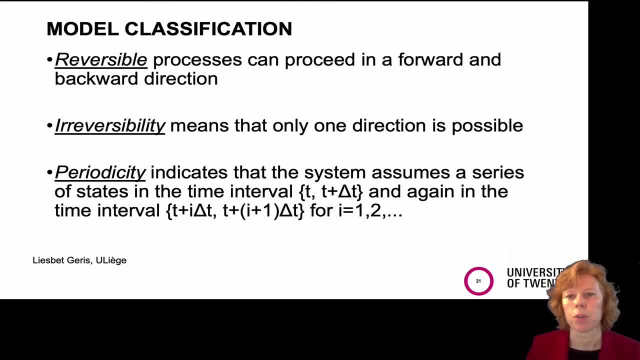 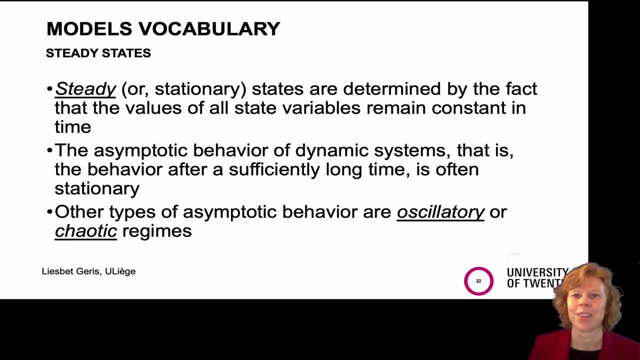 only one direction is possible, and periodic processes in which the system assumes a series of states with specific time intervals. In modeling, as well as in biology, we often talk about steady states. Steady states are reached when the values of all variables remain constant in time. 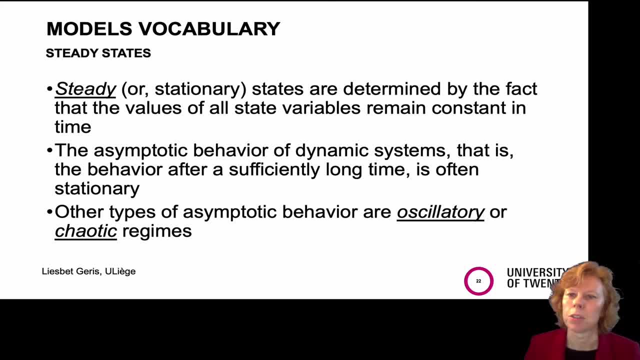 The asymptotic behavior of dynamic systems, or the behavior after a sufficiently long time, is often stationary, so there is no change in values. We do observe other types of asymptotic behavior, such as oscillation or chaotic regimes that continue to exhibit a seemingly unpredictable behavior. 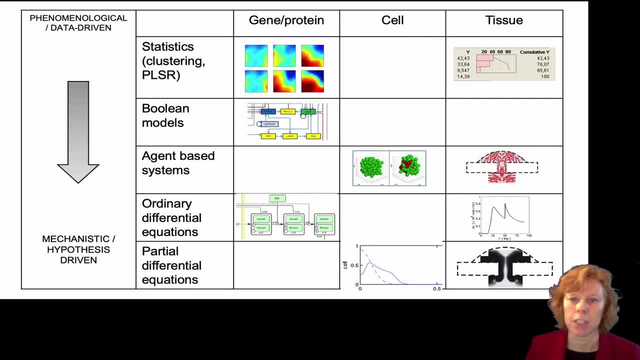 There are many different mathematical tools for investigating system behavior, and they can be arranged from data-driven models, such as statistical models, to mechanistic or hypothesis-driven models, such as ODE models or PDE models. Models of biological systems can be generated at the level of the gene or protein, the cell. 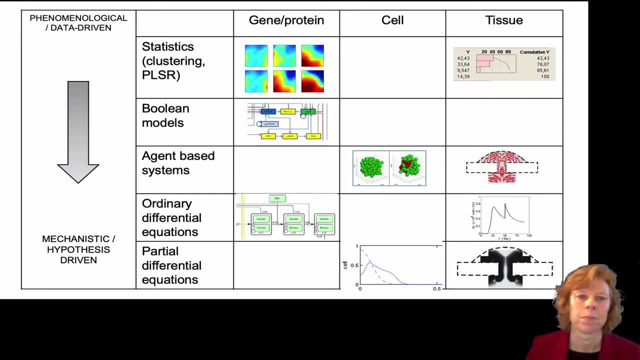 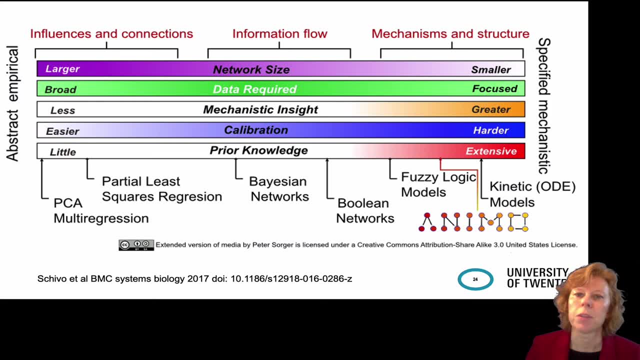 but also as tissue. Thank you, The choice for a good modeling tool very much depends on the system to be studied, the amount of detail that is available and the research question that needs to be answered. For example, if you want to investigate a relatively small network with high precision. 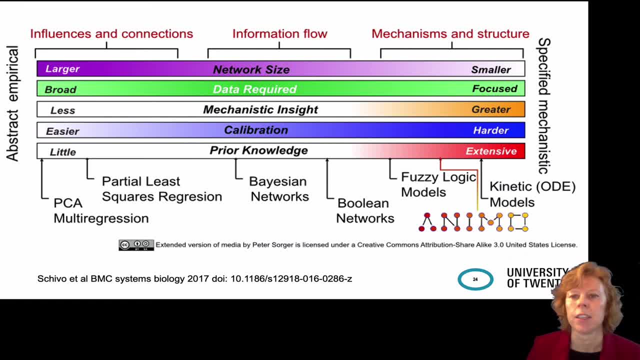 to answer a research question with great mechanistic insight. you want to turn to kinetic models such as ODE, But if you do that, you need to realize that this requires much focused research. Thank you. These models can generate much more complex data and extensive prior knowledge, and that 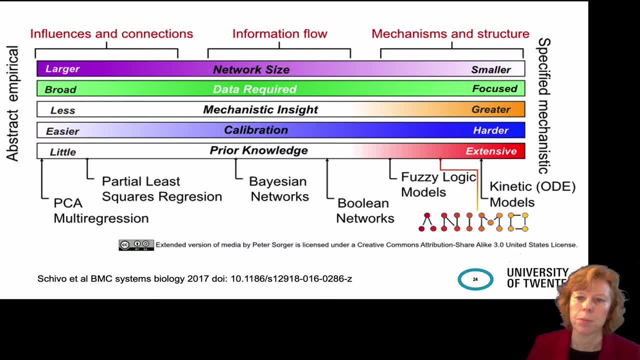 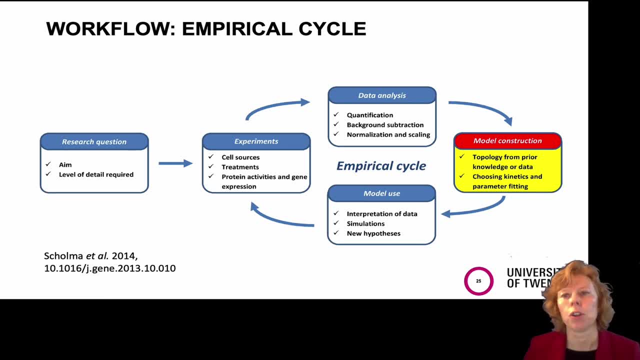 it will be harder to calibrate, Whereas biotin networks can be generated based on less data and less expensive prior knowledge. This may be more suitable for studying larger networks. Computational modeling is used to learn about the system which could be a cell tissue. 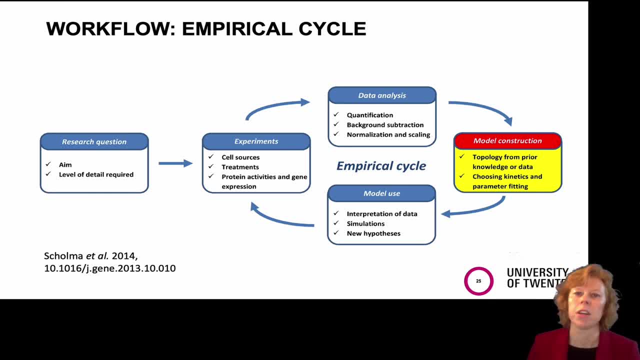 organism. The making of a model is never a goal in itself. The model should be considered an important tool for obtaining more knowledge about a gaining insight into the processes that determine cell and tissue behaviour. To determine what level of detail is required for your model, a clear aim has to be defined. 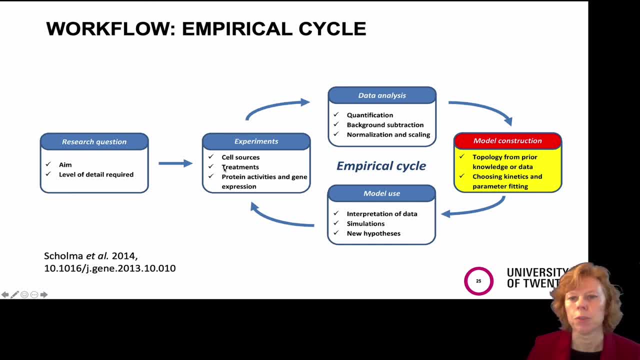 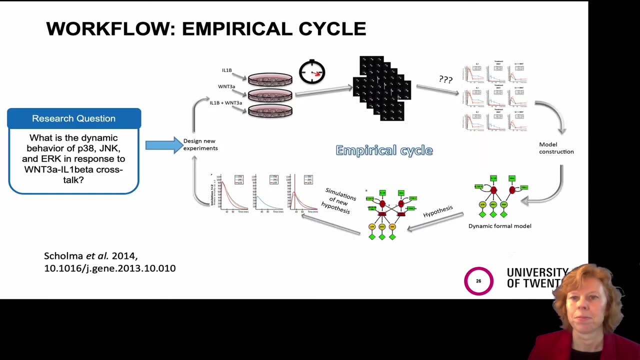 After deciding the aim, one can start at any point of the empirical cycle, in which wet lab experiments are followed by data analysis, model construction and model use, in which new hypotheses can be derived that are subsequently tested in the lab, etc. etc. 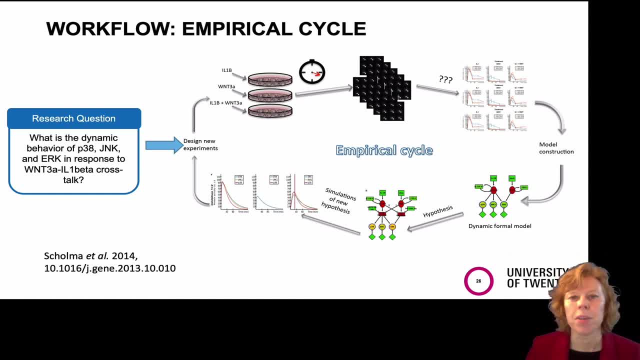 In this example we started with a research question: What is the dynamic behaviour of p38, junk and ERK? in response to Win3A interleukin-1 beta crosstalk, We used wet lab experiments as input. We treated primary articular chondrocytes with either interleukin-1 beta, Win3A or 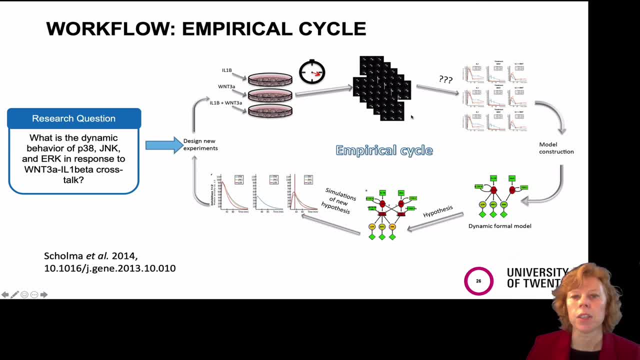 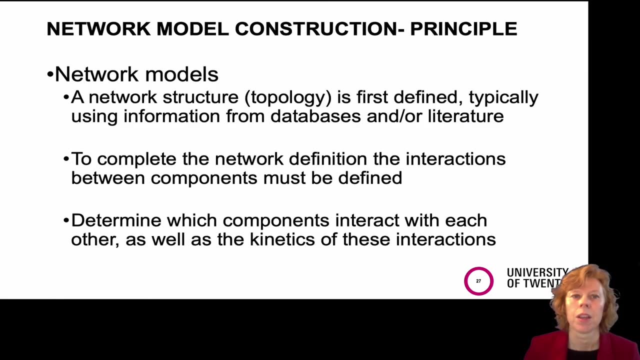 a combination of interleukin-1 beta and Win3A. We then quantified the phosphorylation of p38,, junk and ERK-1. in time, These data were used as input for a dynamic computational model. When generating a network model, different steps are taken. 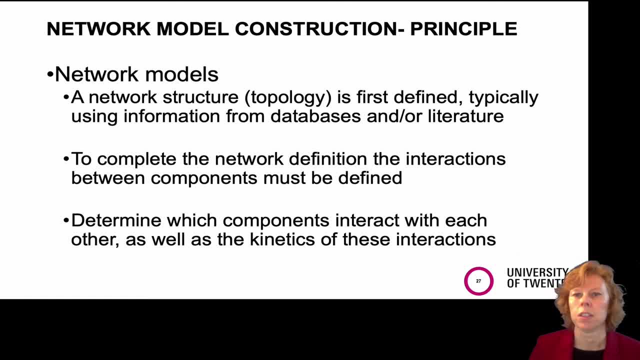 First, a network structure or topology is defined, typically using information from databases and literature To complete the network definition. we use a network structure or topology To complete the network definition. the interactions between components must be defined. One needs then to determine which components interact with each other, as well as the kinetics. 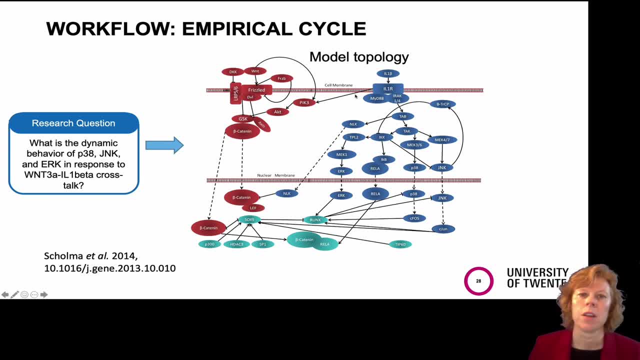 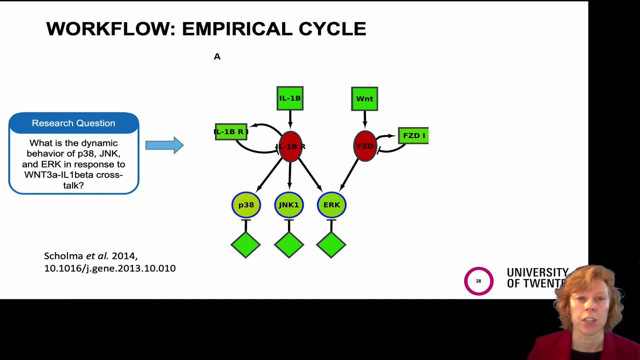 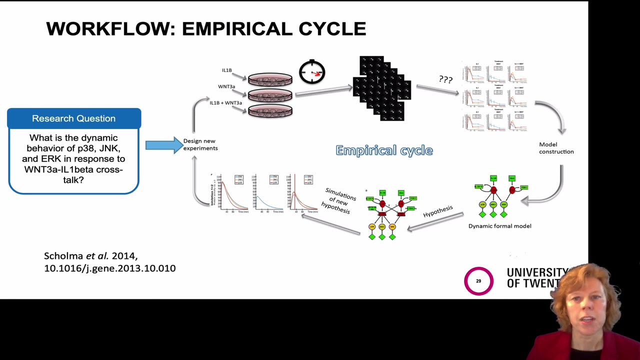 of these interactions. This was our starting model topology for our research question. However, modelling this would be way too much detail for answering our research questions. We therefore simplified the model to the basic interactions. The wetlab data that were generated were used as input for a dynamic computational model. 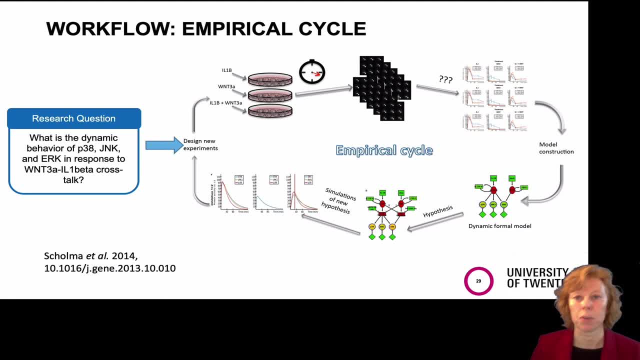 We used this to test two hypotheses, The first one being that wind inhibits interleukin signaling upstream of p38, junk and ERK-2.. And the second hypothesis was that interleukin-1 beta inhibits wind upstream of ERK-1,2.. 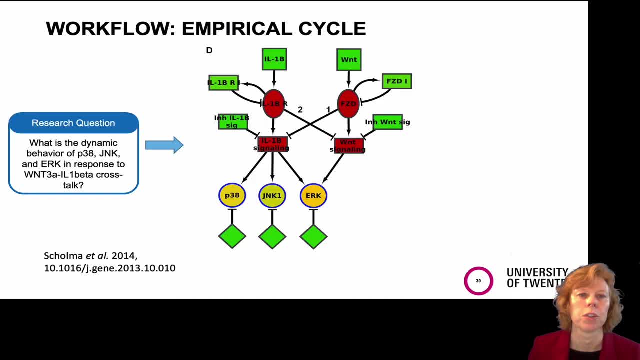 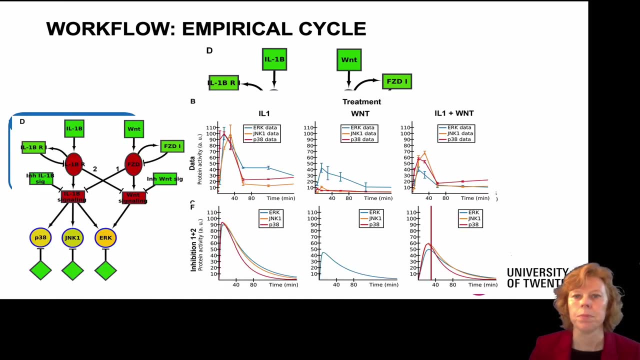 We then tested these hypotheses in the lab and adjusted the model according to the data. So this model, this topology, shows these two hypotheses 1 and 2.. Adjustment of the model to match the in silico experiments with wetlab experiments showed.